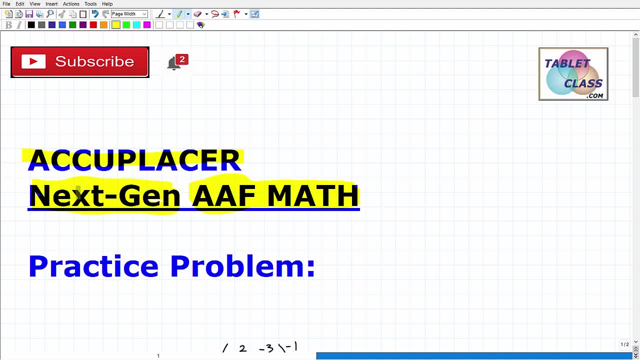 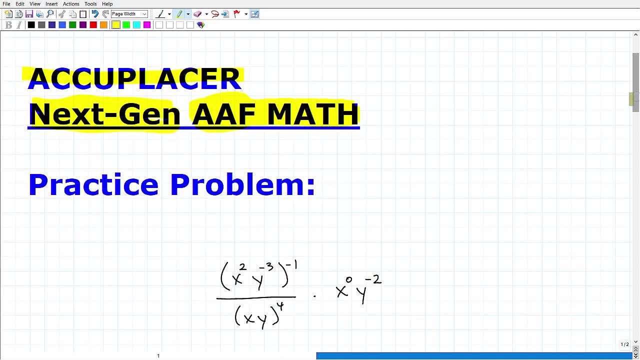 for your current skills and potential. So, anyways, what we're going to do in this video is take a look at a practice problem. They should be able to handle pretty easily if you're fully prepared for the ACCUPLACER Next Generation AAF exam. 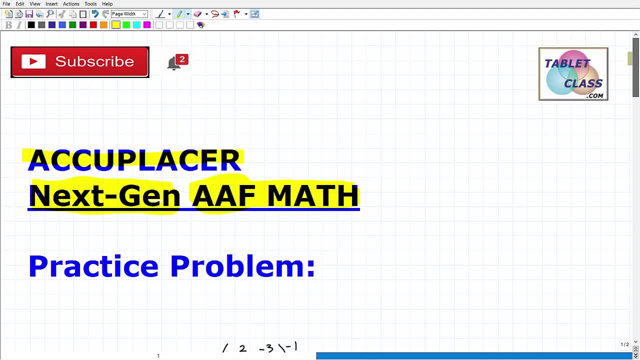 But we'll get to that problem here in a second. But first let me go ahead and introduce myself. My name is John. I'm the founder of Tablet Class Math, also a middle and high school math teacher, And over several years I've constructed many online math courses to include an ACCUPLACER Next Generation AAF test prep course. 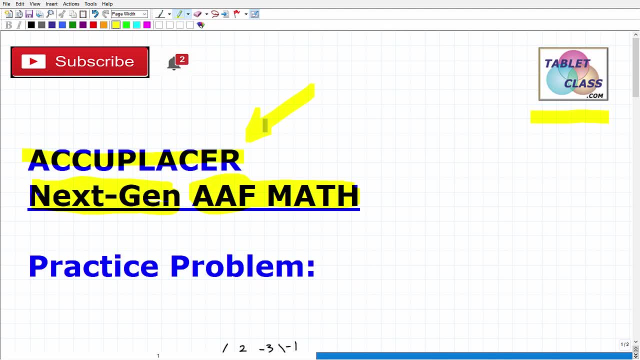 I'm going to leave a link to that in the description of this video. But all my courses are very comprehensive and they've taken me a long time to build. This particular one has been very, very effective. So If you want to check that out again, I'm going to leave the link in the description of this video. 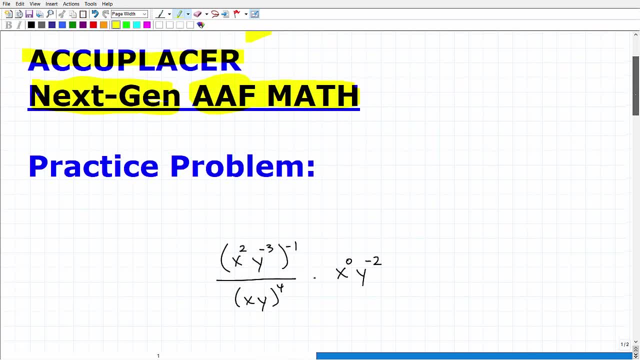 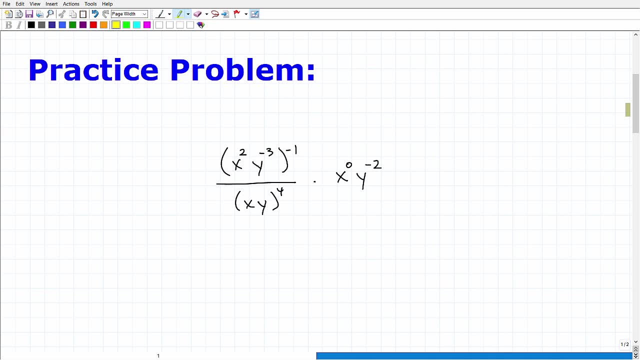 But with that being said, let's get to this problem Now. the way I like to kind of do these videos is one first tell you what the problem is. Then, for those of you out there that think you can do it, you should just try the problem without you know. watching me do the problem. 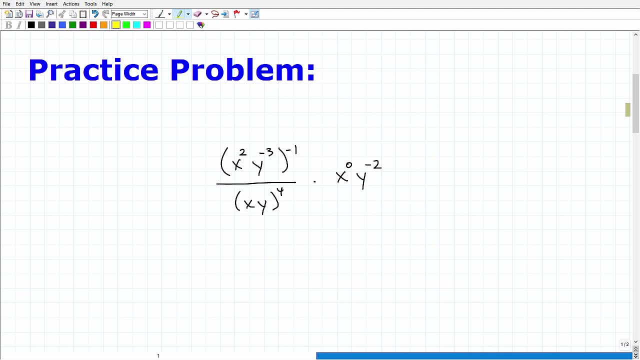 OK, but if you need a little bit of a hint, I'm going to go ahead and give you a hint, And then, of course, I'm going to solve the problem. So if you don't want to hear the hint, Go ahead and pause the video now. 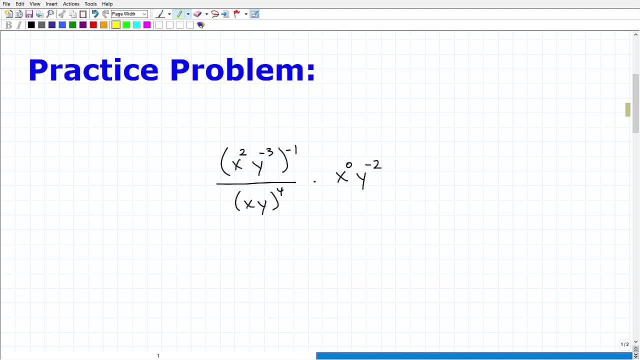 OK, so let's get to this hint, All right. So, first of all, what is the problem? Well, actually, Let me tell you what the problem is. So here I have some powers going on, I have different bases and whatnot. 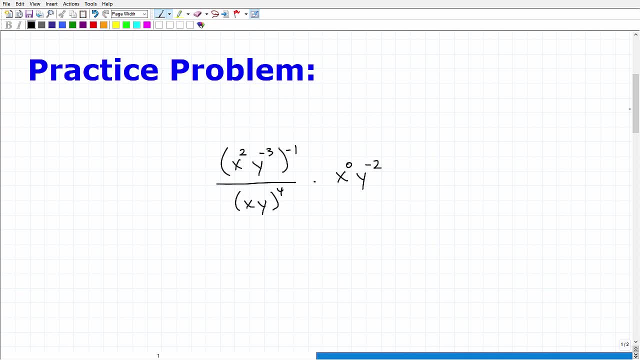 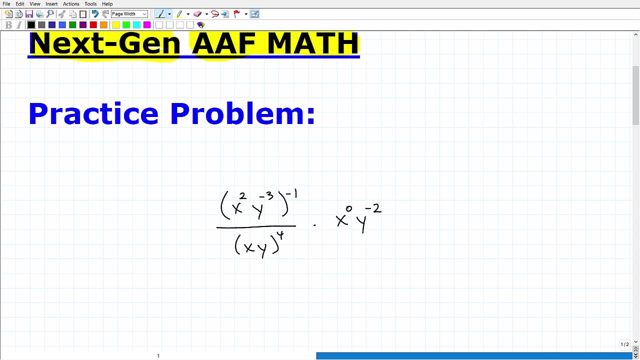 What I want you to do is to simplify. So really I should be more clear about this. What is the problem? So I want you to simplify this expression. OK, so this would be think of it in math, If you have like. 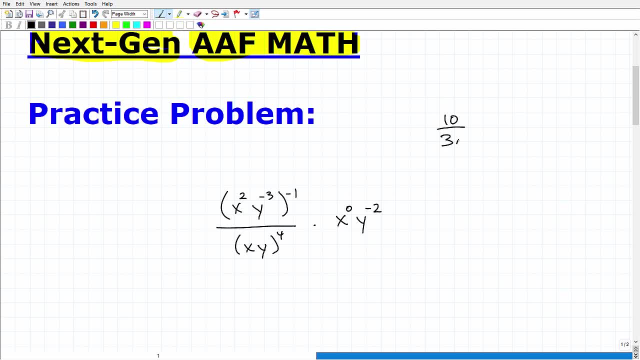 OK, Let's say you had 10 over 30 times the square root of 25.. Right? Would we leave our final answer like this? No, we wouldn't, Right. You want to simplify things. So 10 over 30 is the same thing as one third. 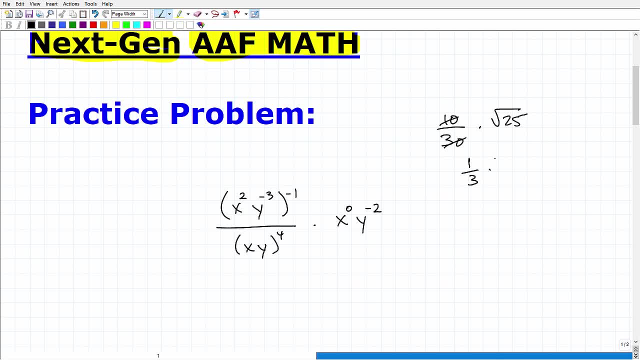 And then the square root of 25 is positive negative five And you can kind of get the idea Right. We don't like to leave things in a non simplified manner, But in mathematics OK, It could be a little bit deceiving when you look at something like this. 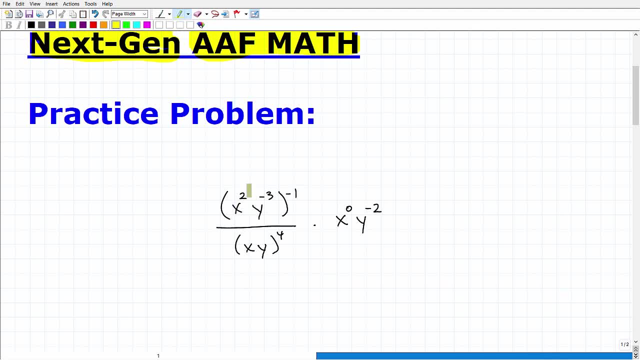 We don't. There's things we can do. We can. We have X's and Y's and exponents, So you can combine this into a much more simpler form. So that's what I want you to do is I want you to simplify this to its fullest extent possible. 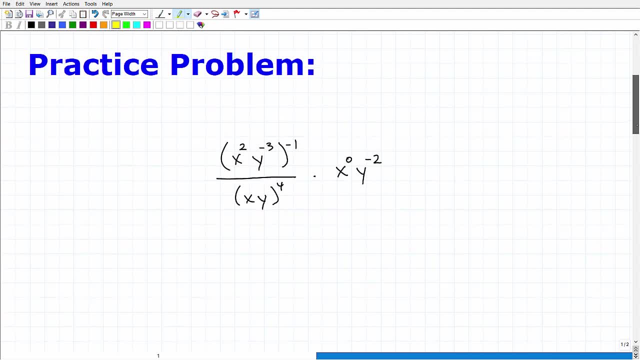 OK. So now here comes the hint. All right. So the hint is: well, what's going on? Well, we have powers and exponents, So you need to recall the rules of powers and exponents. OK, So things like: if I have X squared to the third power, what is the rule here? 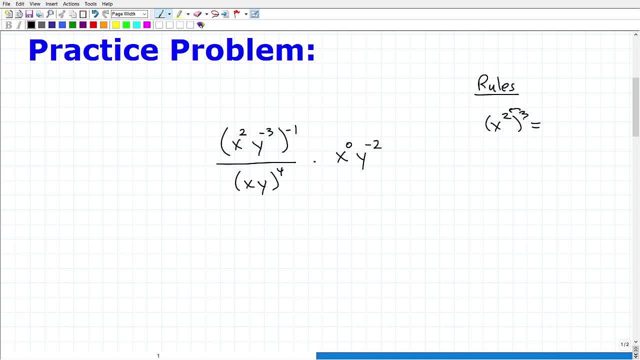 Well, the rule is I just multiply this outer exponent to this inner exponent, So this is X to the sixth, for example. OK, Now what if I had X squared times X, X, Whoops. X to the fifth power. 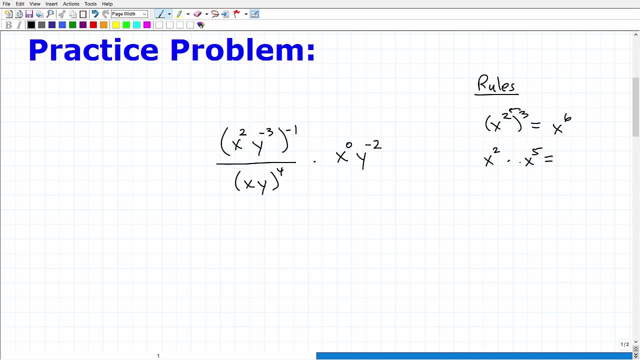 OK, And what do I do there? Well, because the bases are the same, I can add the exponent. So this is X to the seventh. Now you're going to need to know these rules and additional rules. OK, All these rules are very, very important in algebra. 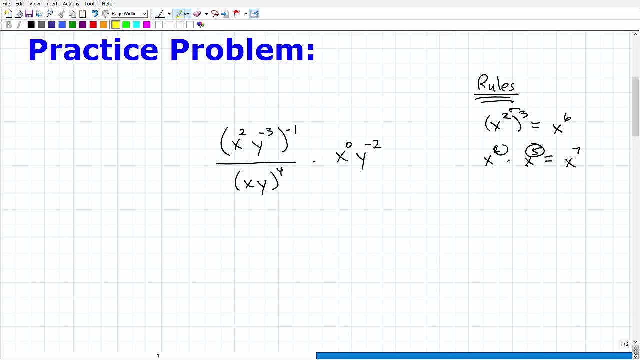 But the hint that I'm kind of driving at here is: these rules are what you're going to have basically have to keep in mind As you manage this problem. Now, there isn't any one particular right set of steps to do this problem. 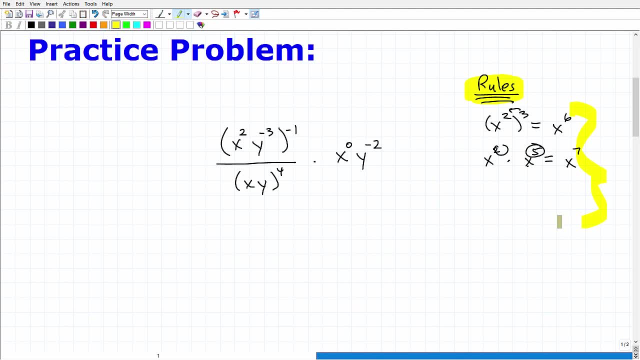 As long as you're doing things that are correct, everybody will eventually get to the right answer. All right, So I'm going to go ahead and solve this now using these rules and other rules, But again, if you forgot the rules, excuse me, don't panic. 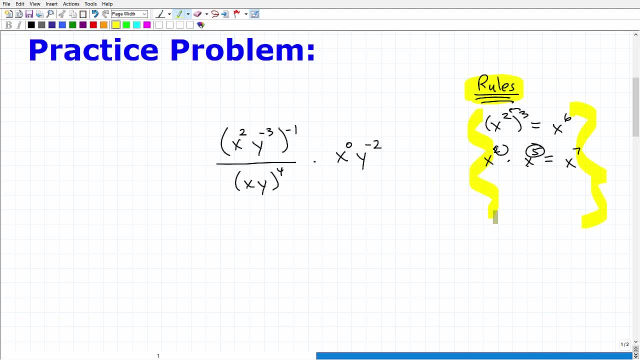 But you're going to have to brush up on these. You know the rules of powers and exponents- Extremely, extremely important, Because in algebra- OK- you're oftentimes dealing with things with exponents Very common. You got to know how to deal with them. 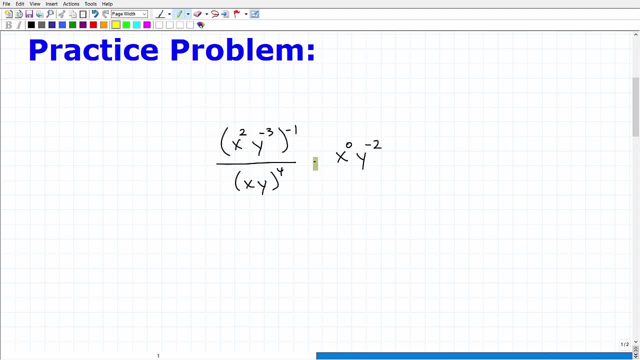 OK, So let's get to it All right. So I have a fraction, And I'm multiplying by this term here, This term over here. Don't let this fake you out And you're like, well, it's not a fraction. 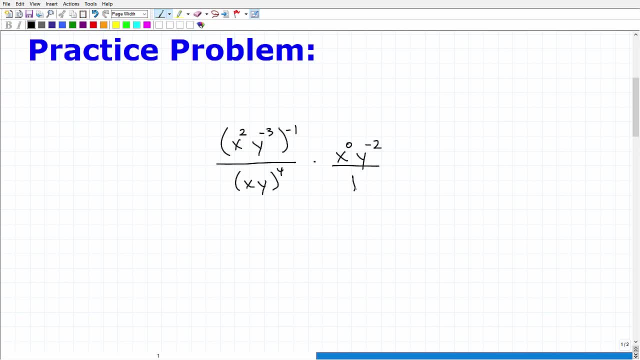 Well, you can always write anything as a fraction, You just put over one. OK, So I have a fraction times another fraction. So how do I deal with that? Well, if I had 2 fifths times, let's say 3 over 4.. 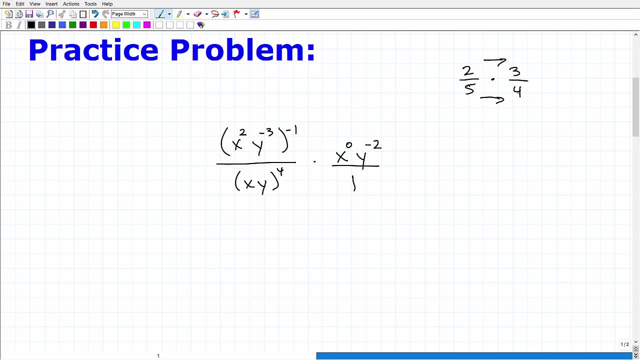 So if I'm multiplying fractions, what do I do? I multiply the respective numerators and denominators, So this would be the same thing as 6 over 20.. Of course, we can simplify, But the point is here that we're going to want to multiply across. 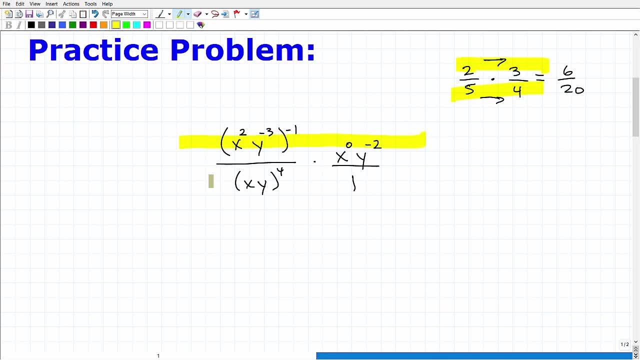 But before we do that, well, let me just finish my thought here. So we're going to be wanting to multiply across, because this is the division of fractions, But before we do that, we can go ahead and start simplifying the individual numerators. 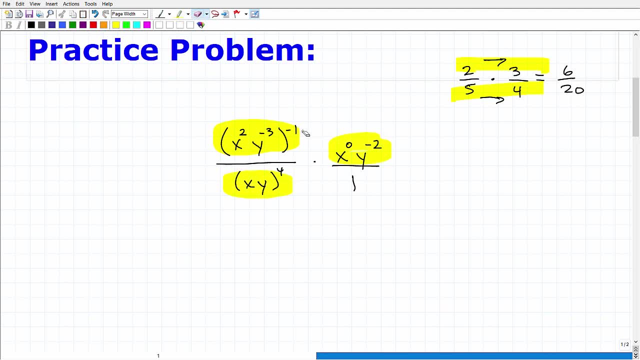 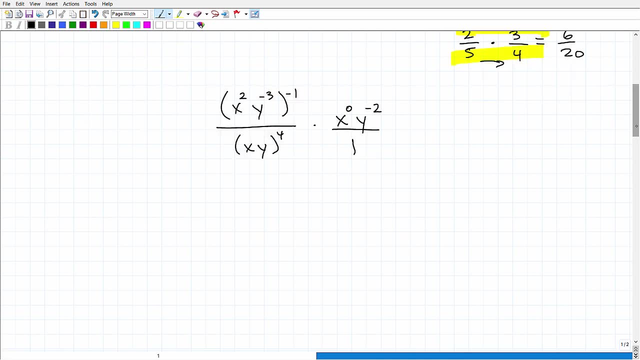 and denominators. So let's get those as simplified as possible, And then we'll go ahead and just start taking some steps to kind of whittle this down into its most simplest form. All right, So let's go ahead and start with this. 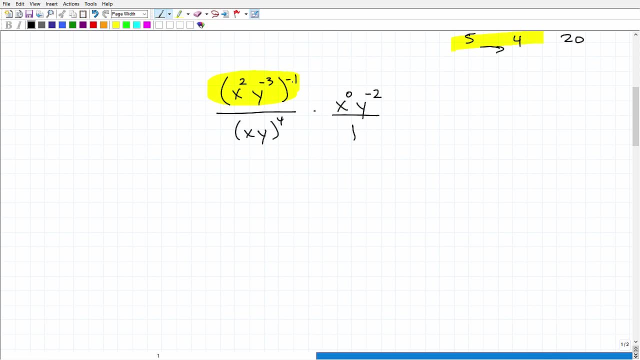 OK, The numerator on this particular fraction. So I can distribute this negative 1 to these exponents. So that's going to give me x to the negative 2.. And then this is y to the negative 3 times negative 1, right, because I'm using a distributive. 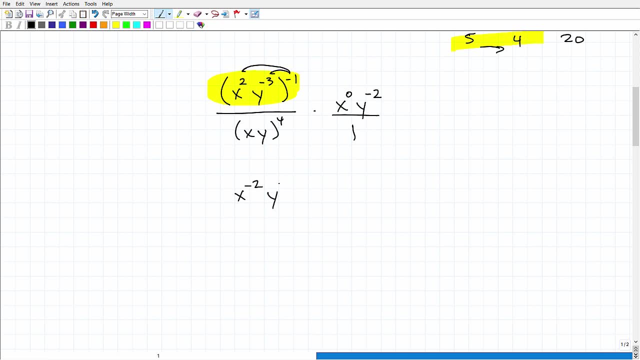 property. So that will be y to the third power, positive. OK, So now let's go ahead and work on this guy. I got this fourth power to the outside of these. Now, inside you just see x and y, But those are both basically x to the first and y to the first. 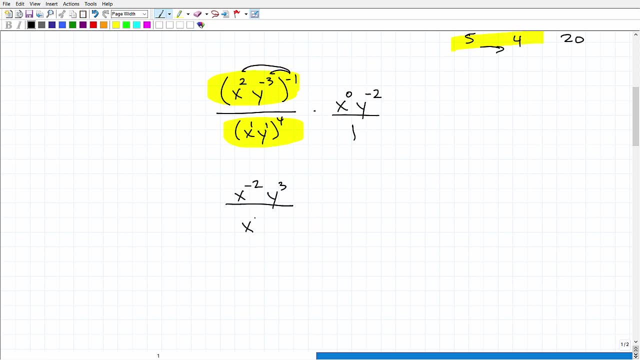 So I can just distribute that 4 in like, so x to the fourth and y to the fourth. And now let's go ahead and work on this a little bit Now. again, this is what I was going to say is: you can continue to try to simplify this. 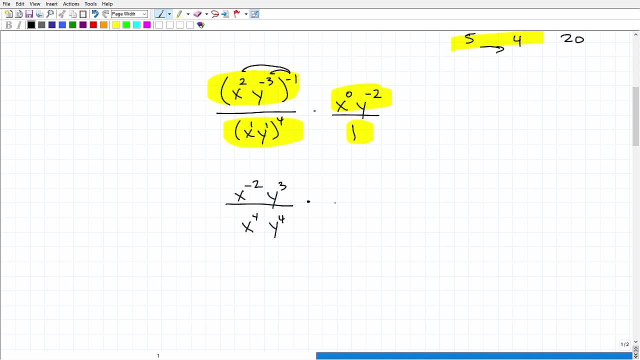 fraction and then work over here, But I'm going to go ahead and just kind of do it in this particular approach. Now here is a question for you: x to the zero power, what is that equal to? All right, So hopefully you remember that anything to the zero power is 1.. 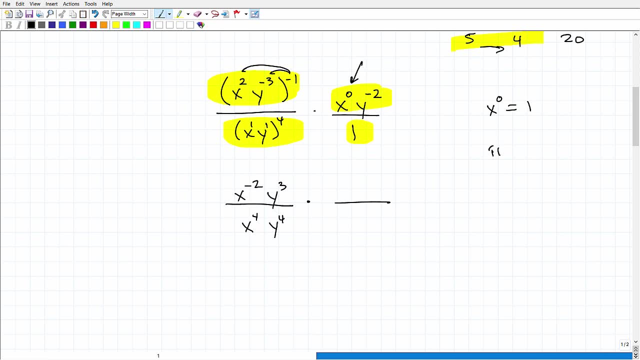 Does it make a difference what you have? You could have pi to the zero power, It's 1.. So anything to zero power is 1.. So this is 1.. And I'm just left with y to the negative 2 then, because this is just going to be 1 times. 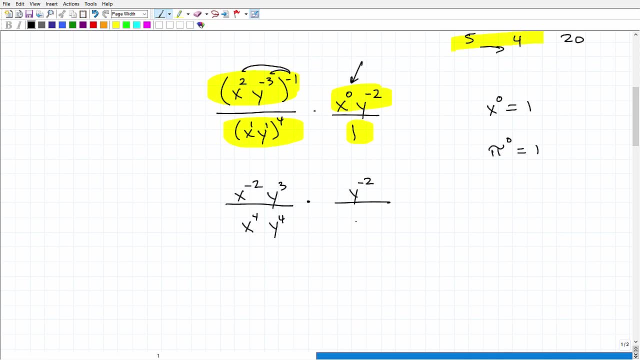 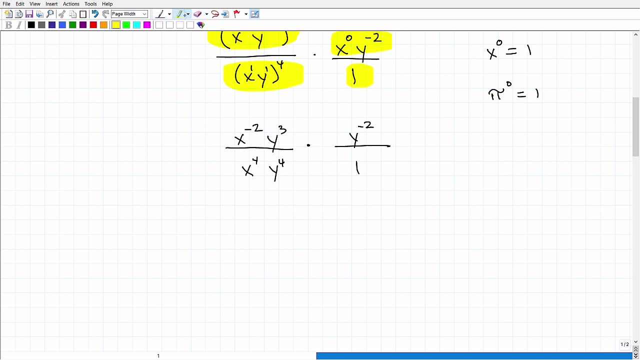 y to the negative 2.. We don't need to write that 1.. And then we'll have this 1 like so. All right, So at this time we can go ahead, and there's different approaches here. We can continue to simplify this fraction, or maybe we could just go ahead and just multiply. 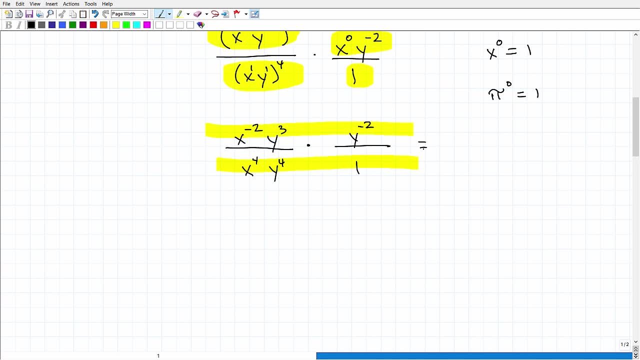 the respective numerators and denominators. So let's go ahead and do that now. So I'm going to take this numerator and I'm going to multiply it by this numerator, So that will be x to the negative. 2 power times, y. cubed times, y squared. 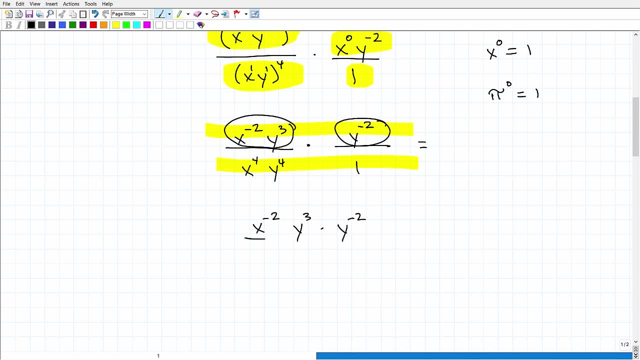 Times y to the negative, 2 over. Now let's go ahead and multiply the denominators. That's easy: x to the fourth, y to the fourth times 1.. So that'll just be x to the fourth, y to the fourth, Okay. 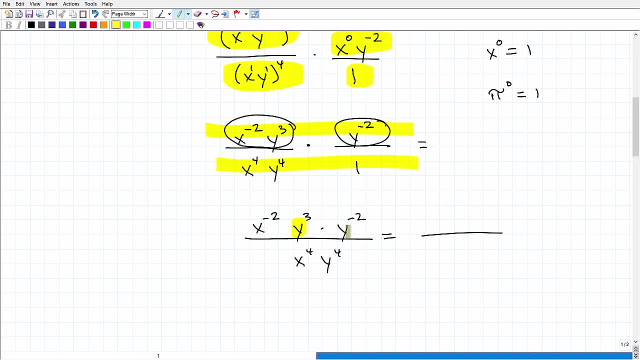 So what do I do now? Well, here, because I have in the numerator. I have two y's. It's the same base. I can add the exponents, So this will be x to the negative 2 power. So 3 plus negative 2 is going to be 1.. 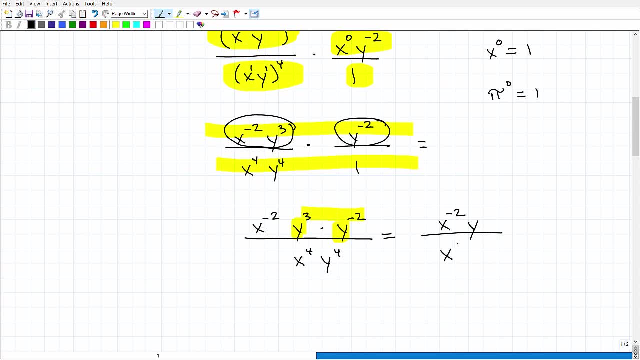 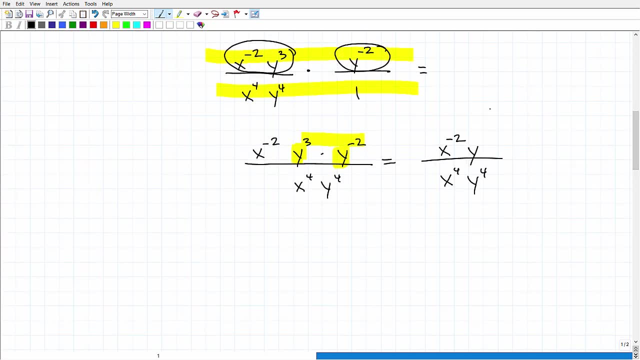 So that's just y. And now I have x to the fourth, y to the fourth. Okay, That's where I'm at right now. Okay, So hopefully let's put a little 1 here, just to make that clear: 3 plus negative 2 is 1.. 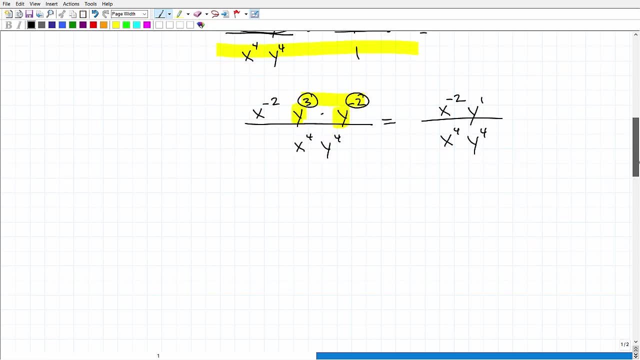 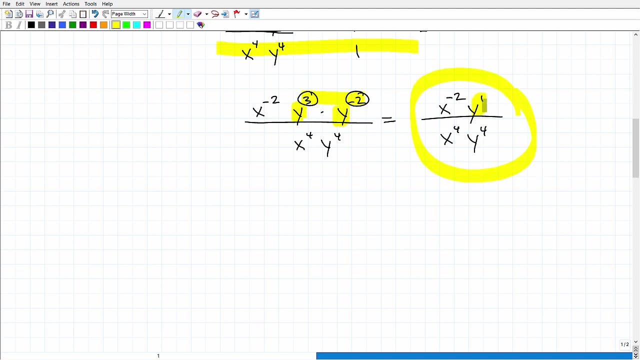 Okay, So we're almost there. Okay, Now let's deal with the y's and we'll leave the x's for the last. Okay, So here I have a y, one y and I have four y's. Let's go ahead and just expand this a little bit. 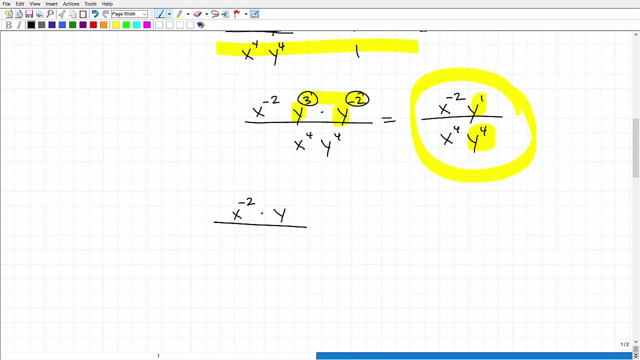 So I have x to the negative, 2 times a, y over x to the fourth, power times y to the fourth, which is the same thing as y times y times y times y. So I can cross cancel one factor, So I'm left with x. 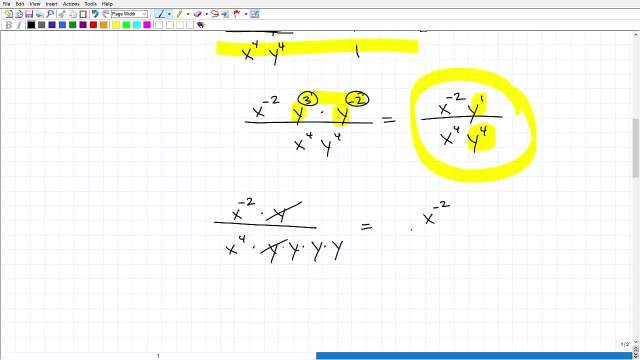 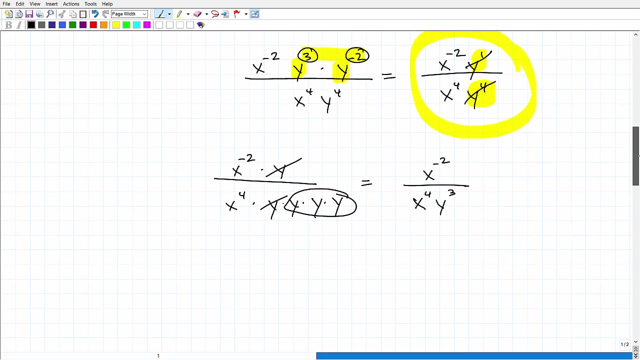 Whoops. x to the negative 2 power Over. x to the fourth y cubed, because one of these y's I was able to cross cancel. Okay, Now I am taking somewhat- I don't want to say shortcuts here. I'm taking shortcuts in the explanation of this for sure, because you know it's hard. 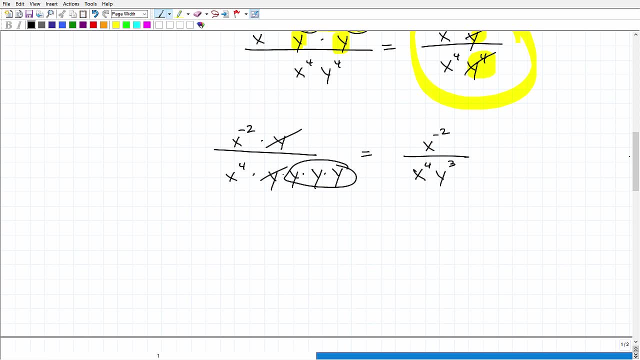 for me to be teaching all these properties. you need to know, you know, as we're doing the problem. Okay, I'm trying to give you, I'm trying to give you a quick explanation of what's going on, But if you're lost here, okay, don't panic. 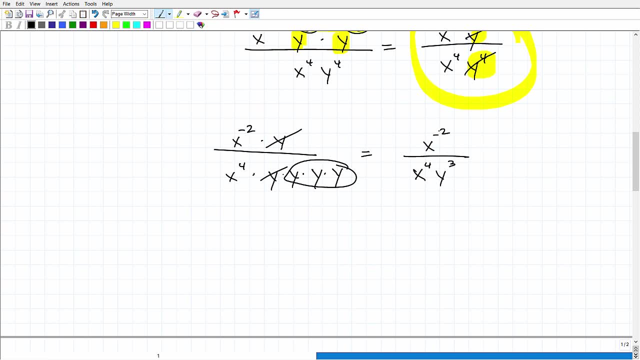 Just make a mental note of what you have to do, All right, So the last thing we have to deal with is we have this x negative 2 and x to the fourth, because you both have between these two powers. they have the same base. 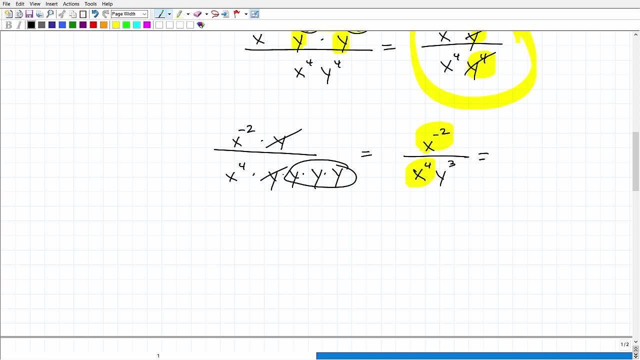 So how do we deal with that? Well, the best way. well, I would say the best way. you have two options here. You can use the division powers of exponent, Which is a to the m over a to the n, and that's equal to a to the m minus n. 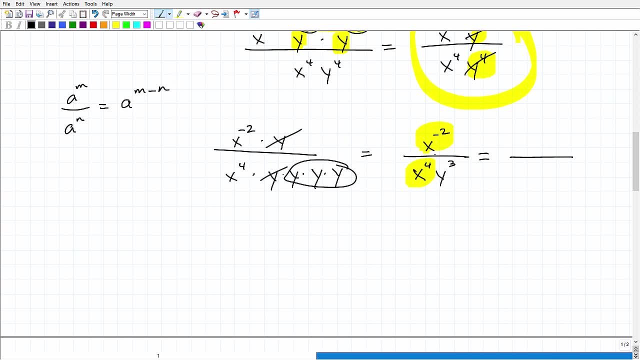 That is the rule. In other words, I can subtract this 4 from this negative 2 minus 4, but I'm not going to go that route. What I'm going to do is I'm going to take this x negative 2 and put it down stairs next. 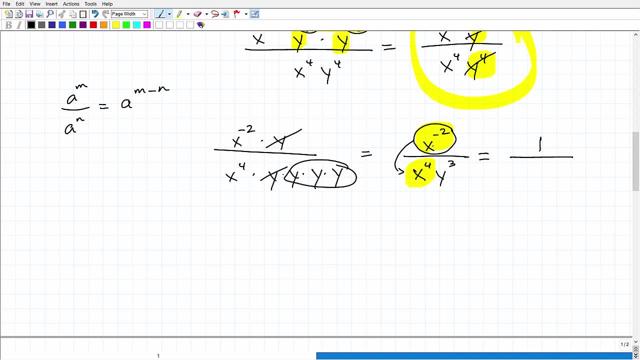 to this, x to the fourth. And I could do that by simply just moving the power down in the denominator, And when I do that, this negative 2 goes away. Now the reason why I did I made this move. Let me go ahead and finish writing the whole thing. 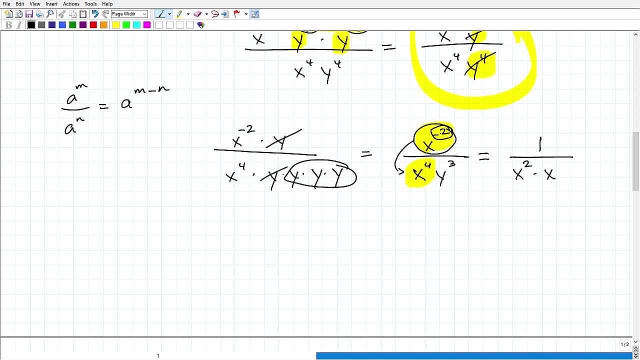 So that's going to be. instead of my x to the negative 2 up in the numerator, I'm putting it down in the denominator. Now I have x to the fourth times y cubed. All right, I'm just putting a little multiplication dots just to make clear that this is multiplication. 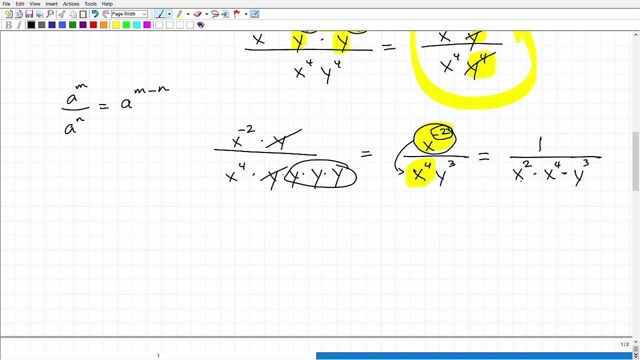 The reason why I did that is because when you're working with powers and exponents, you want to eliminate any negative powers. So this was the option that would have done so. Now again, I'm sure some of you out there if you're not really clear what's going on. 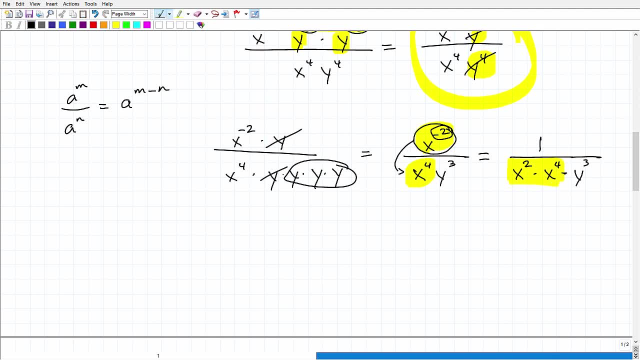 this probably even confused you even more. so, Okay, Again, just use this video as feedback. All right, You're going to. this is, I would say, is more like a basic level, an average level problem. So let's go and finish it up and you can kind of gauge your answer. 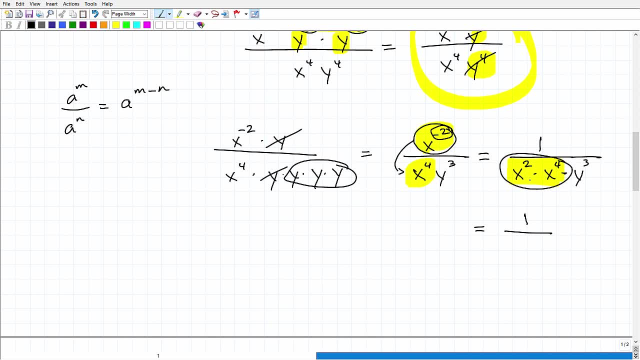 So now they have x squared times x to the fourth in the denominator. I can just add the exponents, So this would be one over x to the sixth, power times y cubed, And that is the final answer. Okay, Now if you had something different that has negative exponents again you want to eliminate. 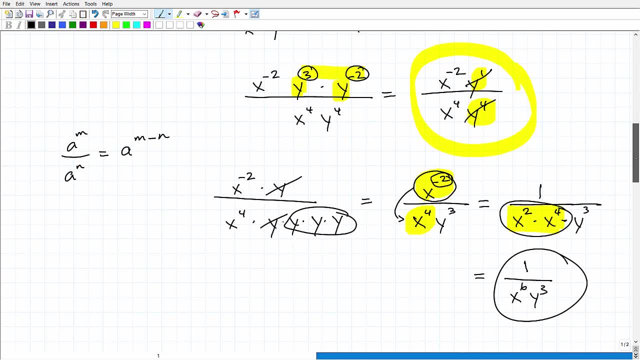 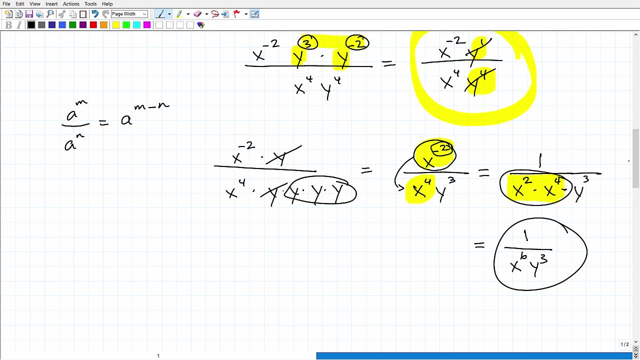 any negative exponents in your expressions, Okay. So if you have negative exponents in the typically in math, we don't do that Typically in math, we don't consider that fully simplified, Okay. So anyways, that is the answer here. 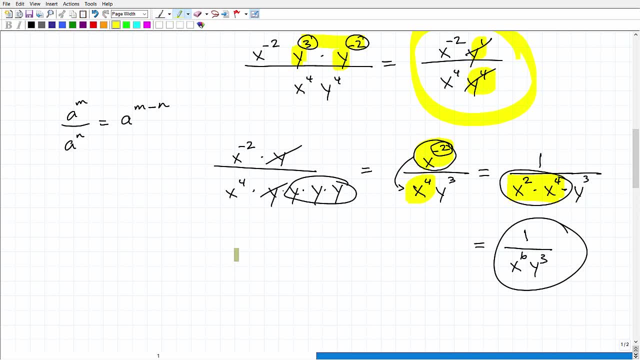 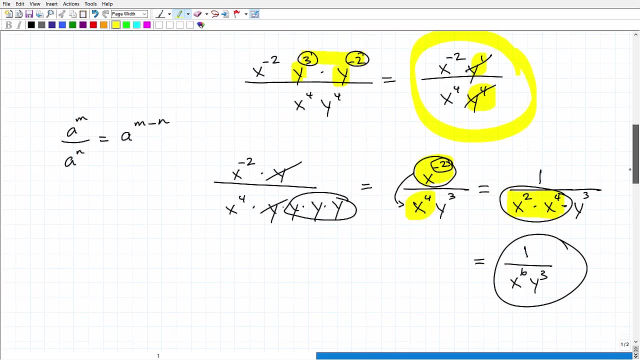 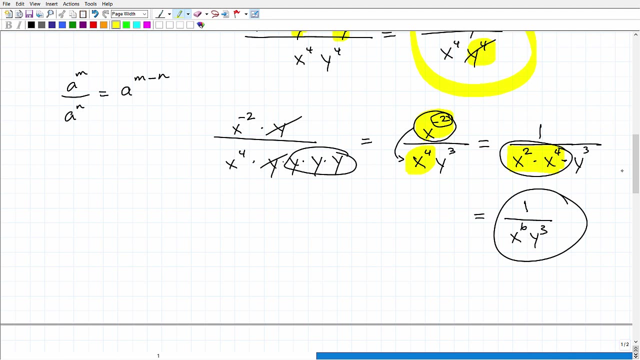 Now if you got this right, I think that's very, very good Okay, Especially if you remembered all this stuff, you know that's definitely a good indication that you're pretty strong with powers and exponents. Of course, there's going to be a lot more. you know problems on the ACCUPLACER AAF outside. 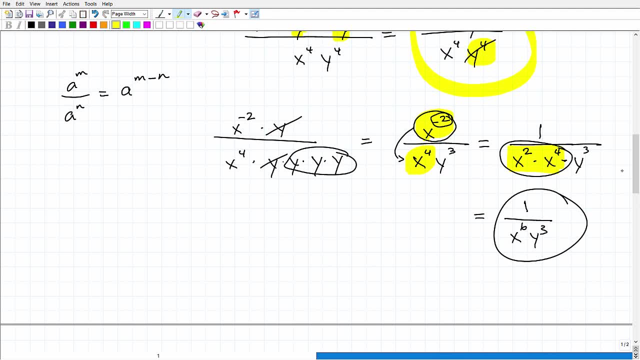 of this, So remember this: If you were lost, don't panic. Okay, And I'm sure a good amount of people watching this video probably struggle with this or forgot how to do it Right? Maybe that's you, Maybe you're like this. 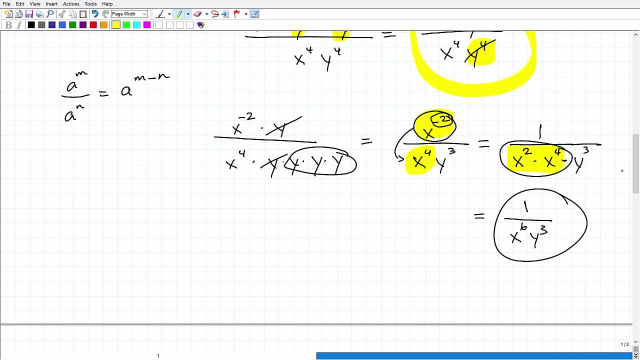 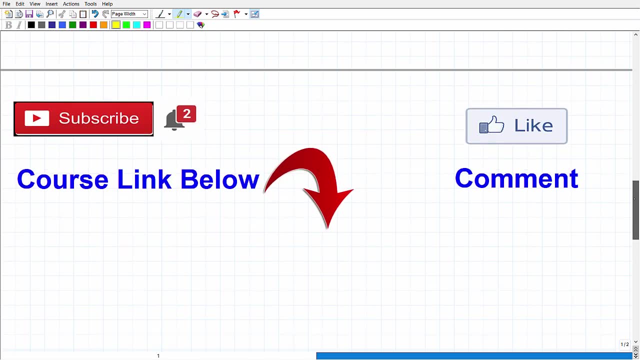 I forgot how to do this, but I do remember, like I do remember how to do it if I kind of have to relearn it, if you will, Right- And that's typically a typical response from a lot of students- Like, oh yeah, I remember how to do that. 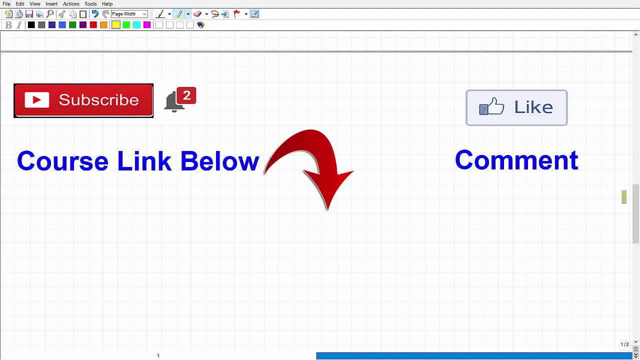 Now here's the thing, though. You can't go into the test and be like: oh, I forgot how to do it. I could do it if I remember how to do it, because the key is you're going to have to. 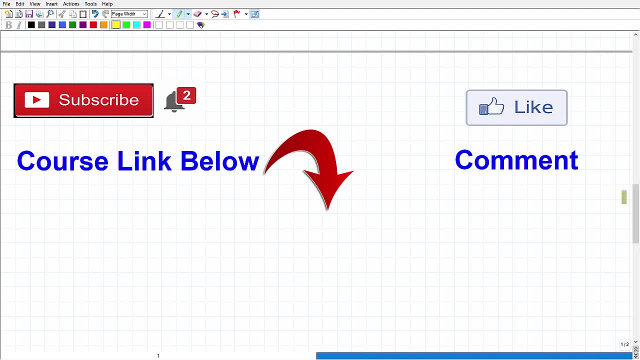 study in advance and you're going to have to cover a lot of different math topics for the ACCUPLACER AAF exam. So do yourself a favor: Study hard before you take the exam so you can place as high as possible and be ready. 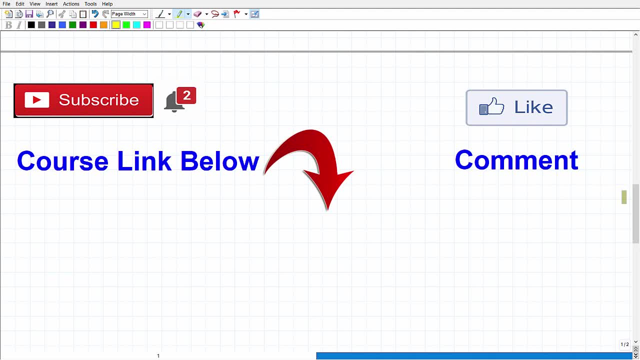 for any subsequent math class that you're going to be taking. So again, just going to remind you that, if you like my teaching style, I want to check out my ACCUPLACER, My ACCUPLACER AAF math test prep course. 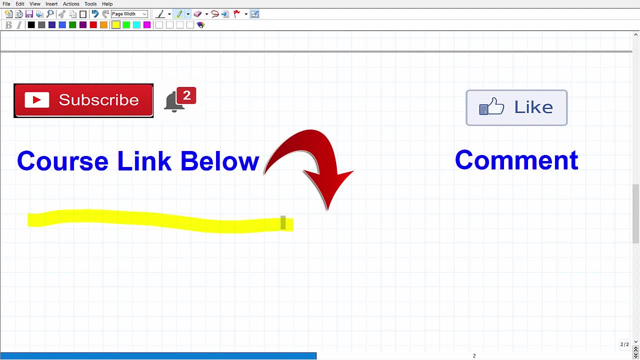 I'm going to leave the link to that in the description of this video- Extremely comprehensive. If you're new to my YouTube channel, I've been on YouTube for a good 12 years at the time of this video, So I already have hundreds of videos on my channel that could help you out. 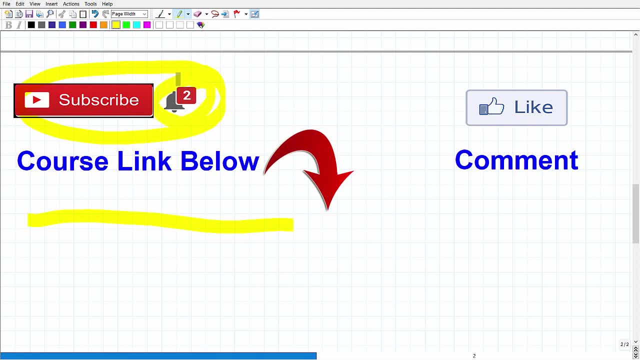 And I'm posting stuff all the time, So hopefully consider subscribing If you like the video. definitely appreciate a thumbs up and leave me some feedback. What was, you know, your highest math class in high school? Are you coming? Are you been away from school? 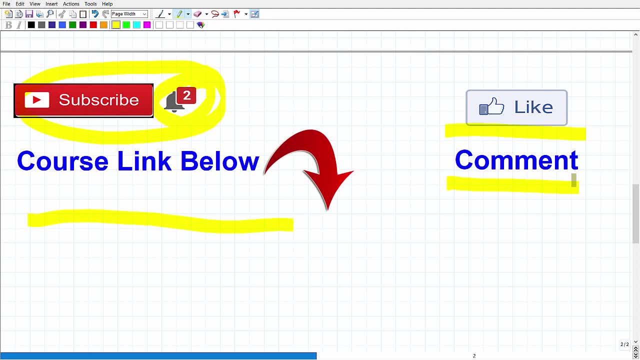 Are you coming out of like a career or you know how you know? maybe you've been away from high school for 10 years, maybe 20 years going back to school, but maybe you're just you know, going right from high school into college. 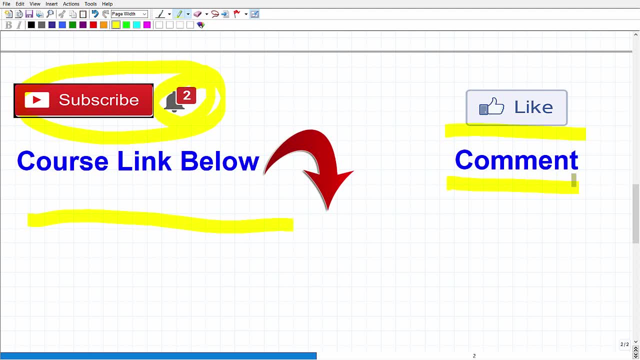 So let me see feedback. Do you like math? Do you don't like math? Yeah, But I always like to kind of say is that I would a good majority of the people out there I find, do not like math as much. Okay,